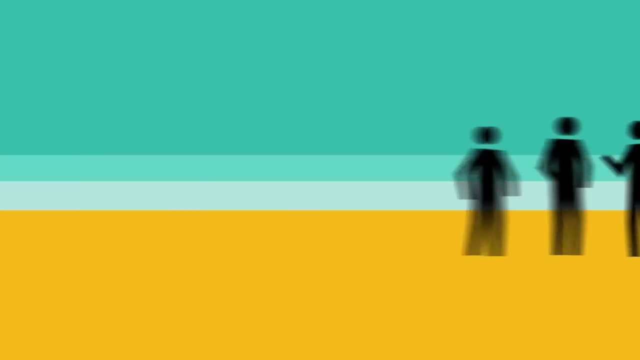 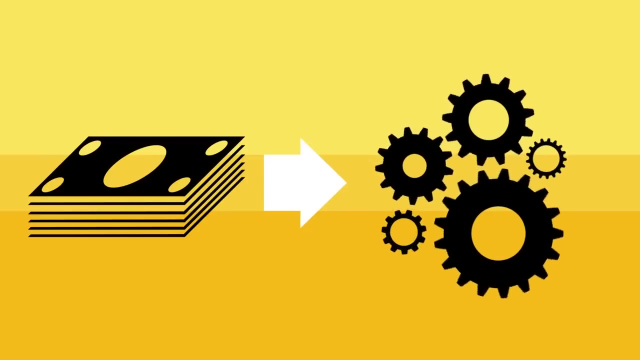 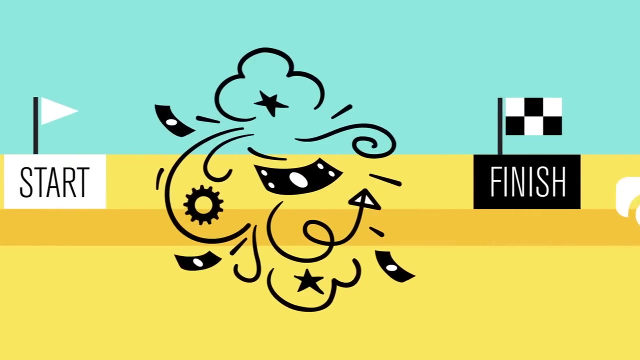 You're looking to offer your customers a safe and easy way to pay online. Since all payment processors aren't created equal, it's a really good idea to know the ins and outs of how an online payment functions, from start to finish, so you can avoid pitfalls and make the most effective choice to protect and grow your business. 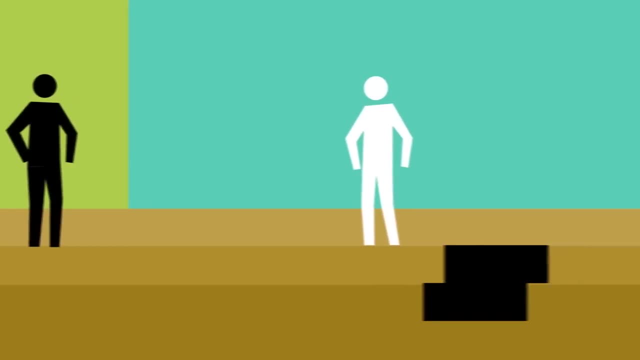 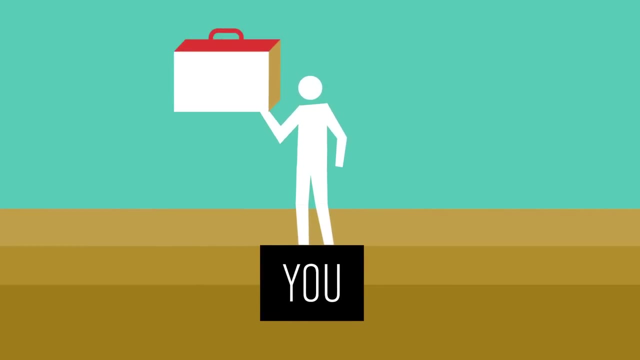 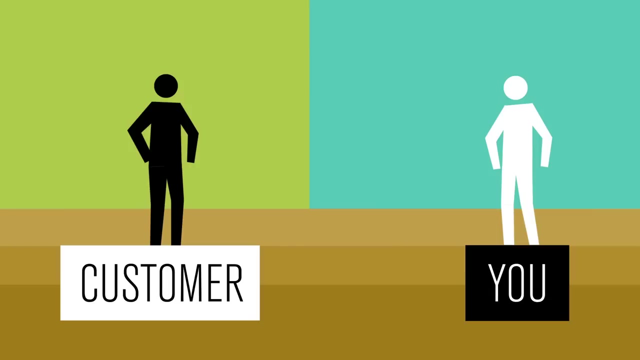 The main players in an online payment are you and your customer. To accept credit cards from customers, you'll need a couple of things: An internet merchant account and a payment gateway. On top of that, you can also choose to include an alternative payment method like PayPal. 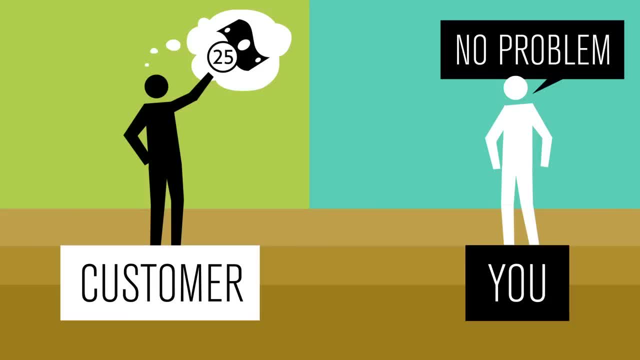 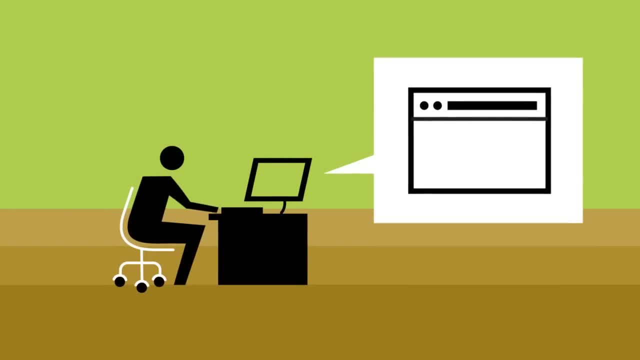 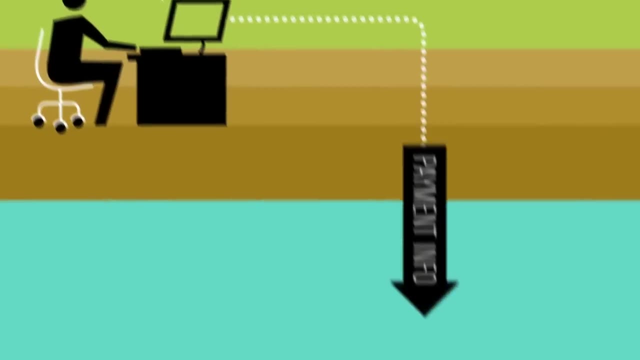 to service those customers who shy away from using credit cards. Once those pieces are in place, here's what happens next. A customer makes a purchase from your checkout page by submitting their payment information. That information is then sent to your account. That information is then sent to the payment gateway. 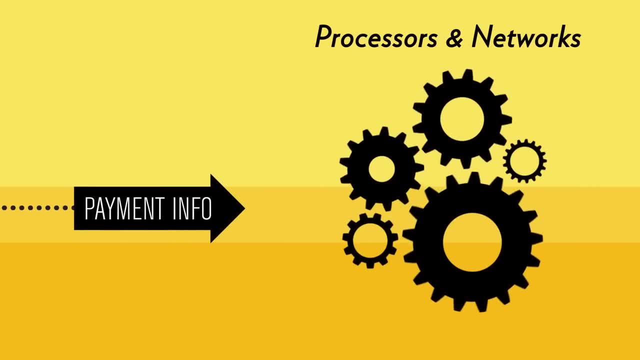 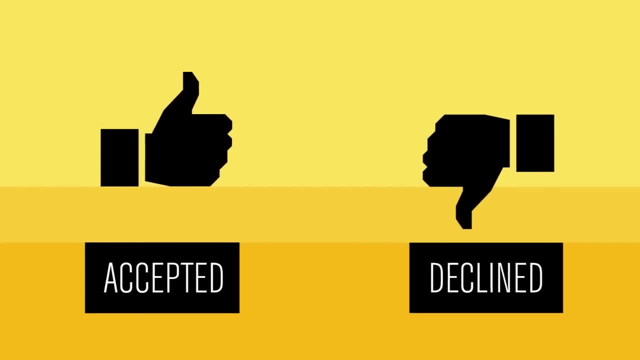 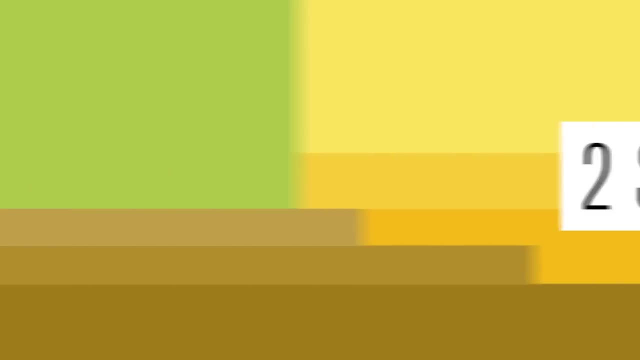 The gateway then encrypts the payment information and shuttles it to a series of approved payment processors and networks for authorization, where the payment is either accepted or declined. That decision then shoots back to your customer And all that flurry of activity takes place in about two seconds. 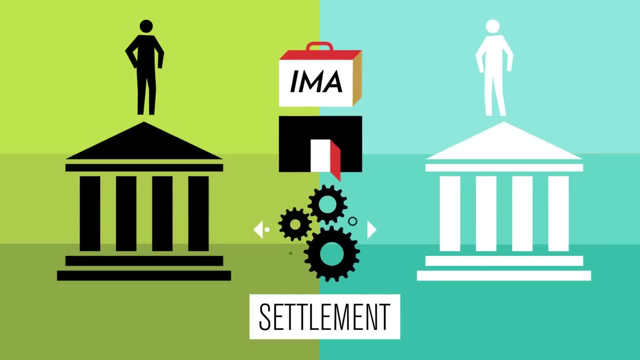 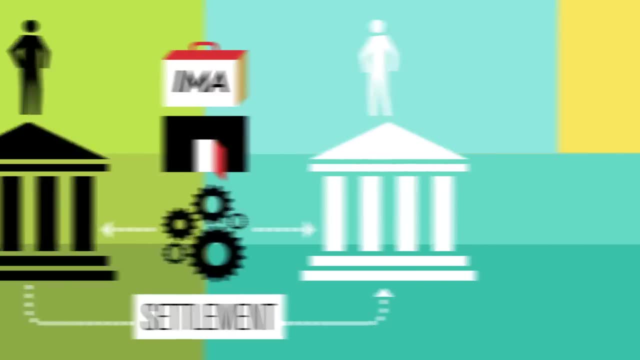 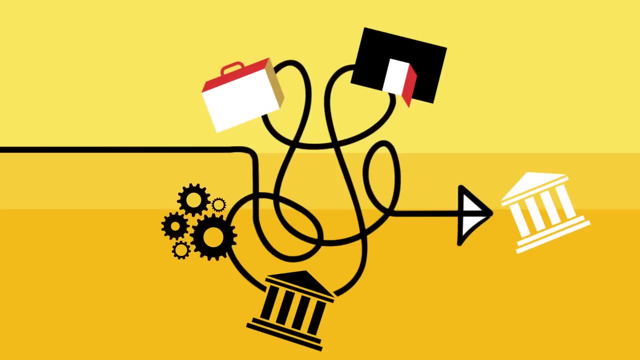 The final step happens after the gateway sends the transaction to the payment processors and the money is transferred from the customer's bank into your account. So, as you've seen, a payment moves through several parties, often with varying providers for each transaction, Since things can get really complex really fast. some payment solutions make things easier to manage. 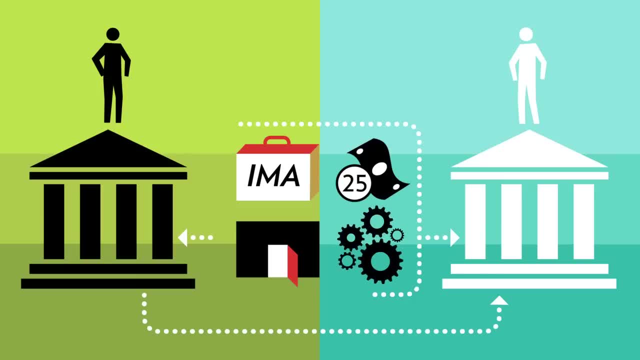 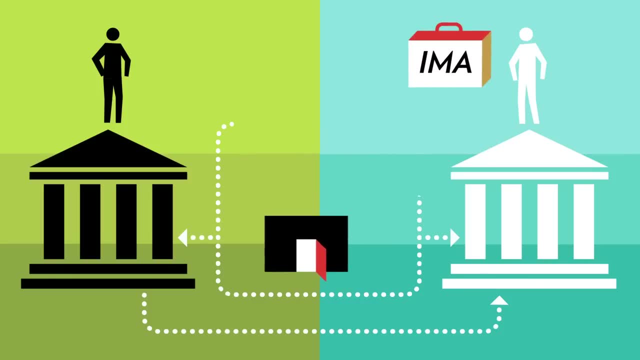 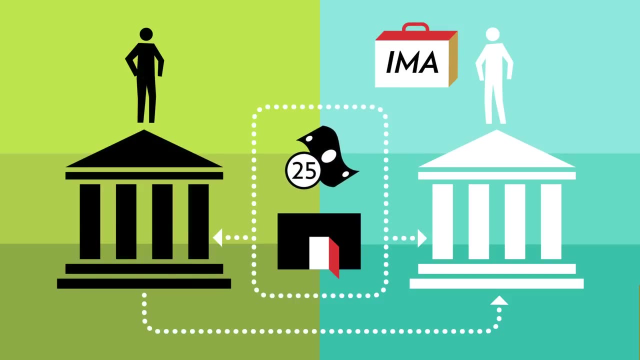 by offering everything you need bundled together into an all-in-one solution. If you already have an internet merchant account, some solutions allow you to use a gateway to accept credit cards and offer the option to add alternative payment methods. There are, in fact, all kinds of different solutions out there.